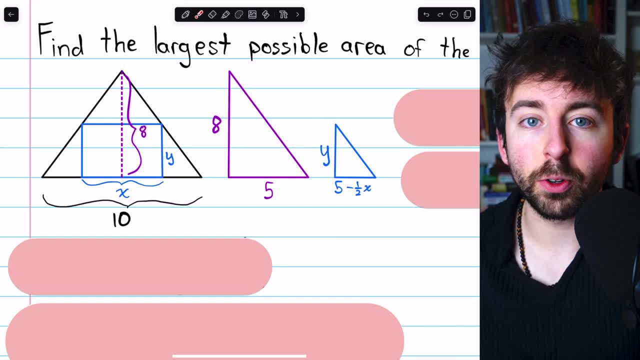 A couple other things we should justify about our similar triangle picture. We know the triangles are similar. How do we know that this base of the big triangle is actually half the base of the larger isosceles triangle? Well, it's pretty easy to see that these two halves. 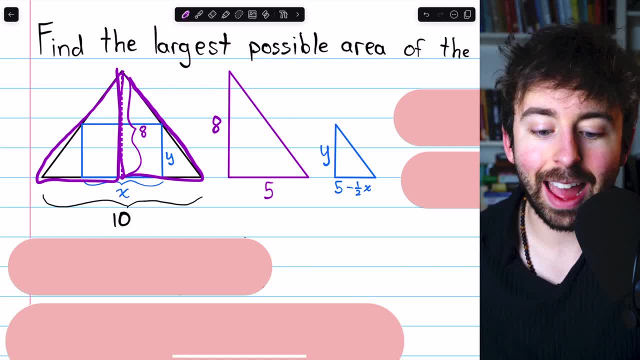 are indeed congruent. We can use angle-angle-side to see that By the isosceles triangle theorem, this angle is congruent to this one. This is a perpendicular because it's the height, and so this angle is congruent to this one. And then, of course, both halves share this side. 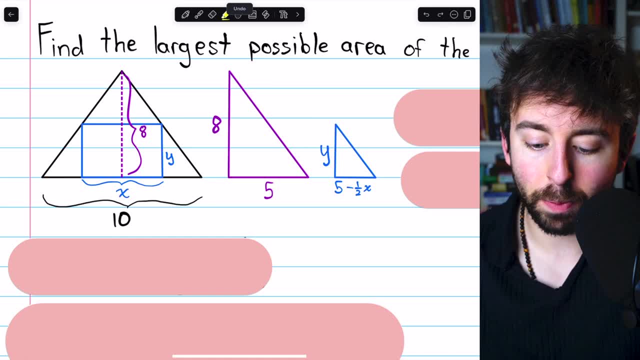 so they are congruent by angle-angle-side. So the perpendicular did cut the isosceles in half, so this base is half of the total base. That's how we know it's five. Now how do we know? the base of this smaller triangle is five minus half x. Well, 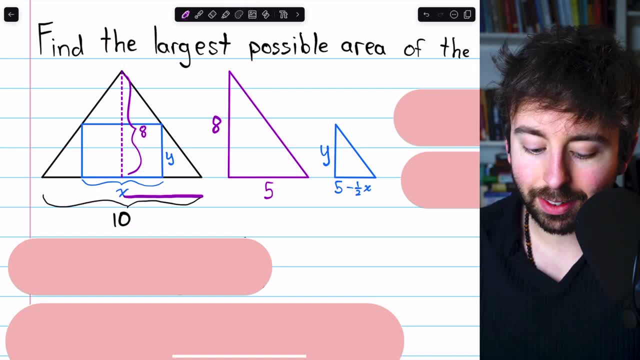 that's because it's this distance minus this distance. This distance we just showed is five. As for this distance, which is half the base of the rectangle, we know that's half the total base of the rectangle because this triangle up here, 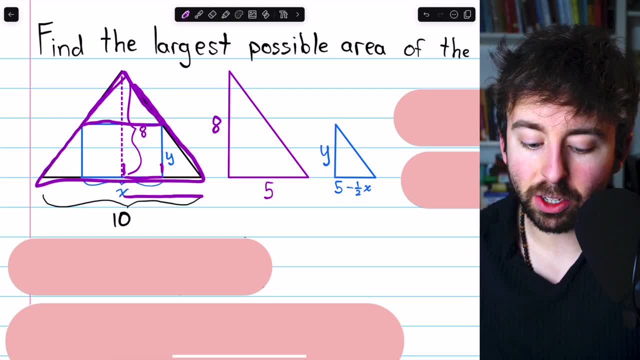 this little one must be similar to the big triangle. So if this perpendicular cuts the big triangle in half, it also cuts this small triangle in half, which means this piece is congruent to this piece. So we know that this piece is congruent to this piece. So we know that this 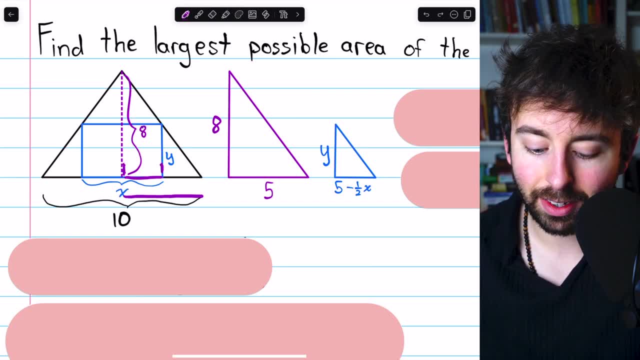 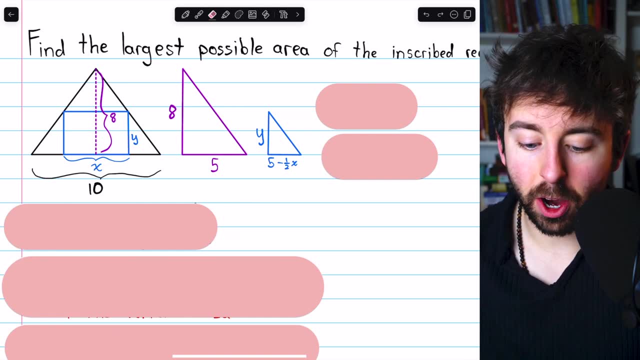 indeed, this guy here is half x, So this distance is 5 minus half x. Now we can really get on with the algebra, Because these triangles are similar and we know what their dimensions are. we know that 8 to 5,. the ratio of the height to the base must be equal to y to 5 minus half x. the ratio of 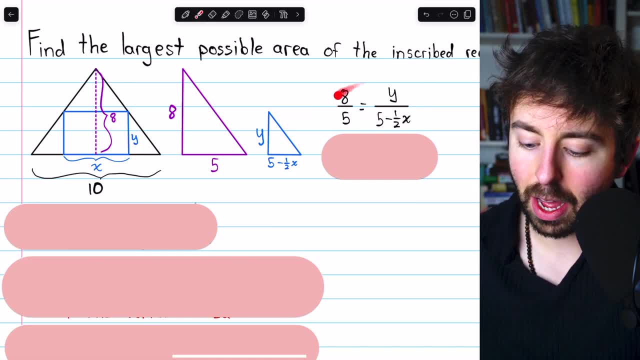 the height to the base, because they are similar triangles. So 8 to 5 equals y over 5 minus half x. Now we can solve this equation for y by multiplying both sides by 5 minus half x, 8 fifths times 5 is 8, and 8 fifths times minus half x is minus 4 fifths x. So we've now expressed: 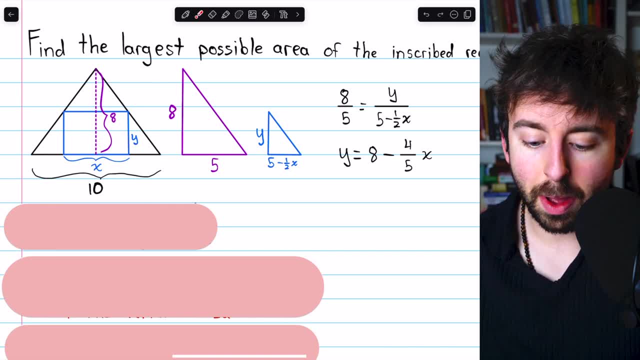 y in terms of x. This is useful because, remember, we're trying to maximize the height to the base because they are similar triangles. So 8 to 5 equals y over 5 minus half x. This is the area of this inscribed rectangle and we can express that area as xy. That's base. 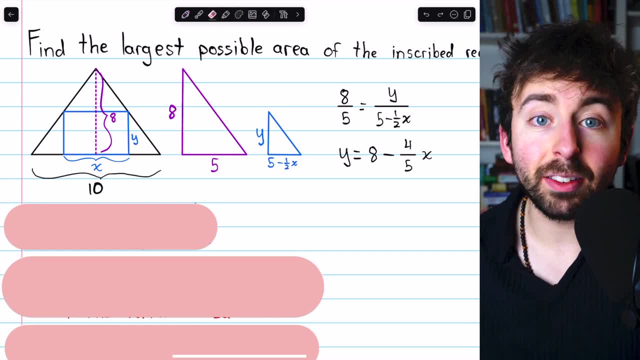 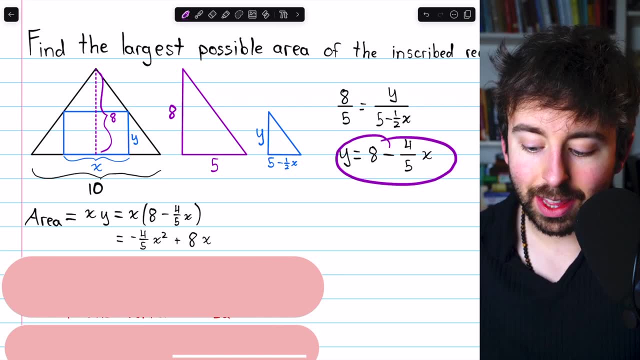 times height. That's a little bit difficult to work with, though, because it has two variables, x and y, But now we know what y is in terms of x, So the area we're trying to maximize is xy. but we know y is 8 minus 4 fifths x, So the area is x times 8 minus 4 fifths x. 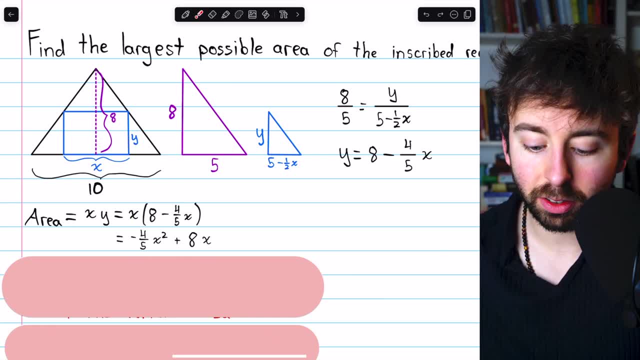 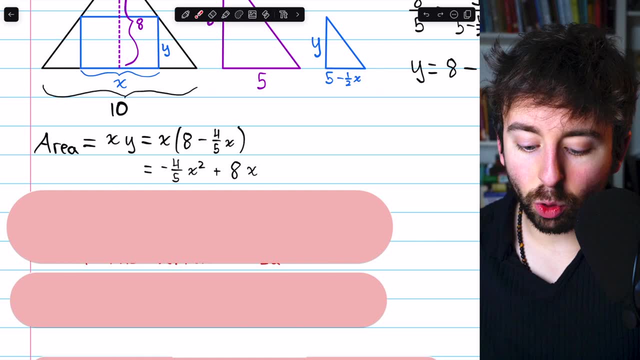 Distributing the x and putting the squared term first, we have minus 4 fifths x squared plus 8x. The question then is: where is this taking on its maximum value, this area of the inscribed rectangle? That's actually a pretty easy question to answer because, you should notice, this is a 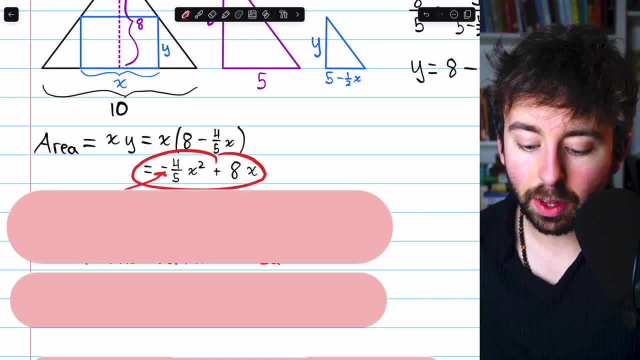 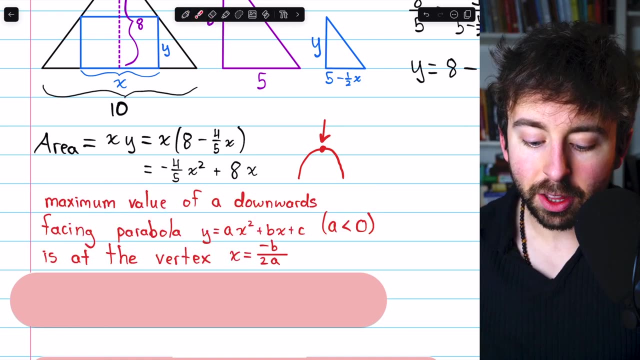 quadratic function where the leading coefficient is negative, which means its graph is a downwards facing parabola and the Maximum of a downwards facing parabola is at the vertex. And there is a simple formula to find the vertex, The maximum value of a downwards facing parabola. if we were to write it like this: where? 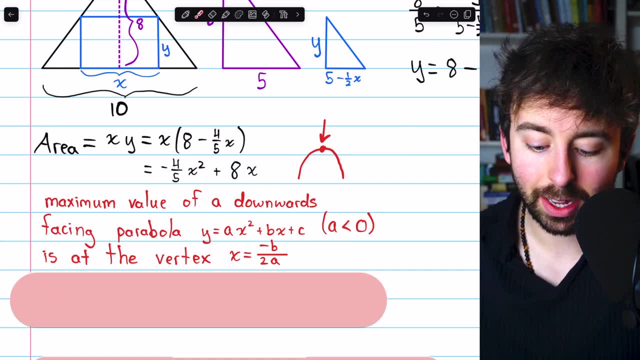 a again is negative because it's a downwards facing parabola, just like our example here. the maximum is at the vertex where x equals negative b over 2a. So we just have to apply that to our situation: Negative 8 over 2a. 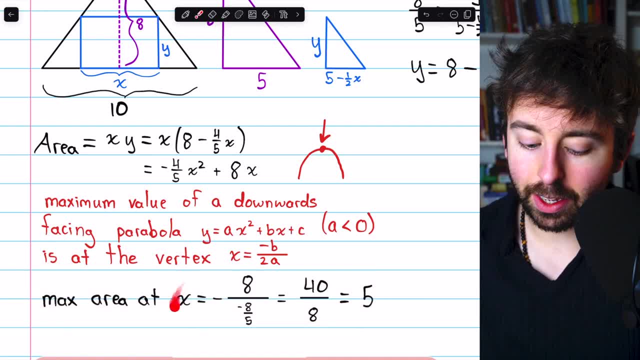 2 times a. that leading coefficient- And there it is, Our maximum area- will occur at the vertex where x is negative b, that's 8, the coefficient of the linear term divided by 2a. a is negative 4 fifths, so 2a is negative 8 fifths. If we evaluate this, we get 40 over 8, which equals 5..